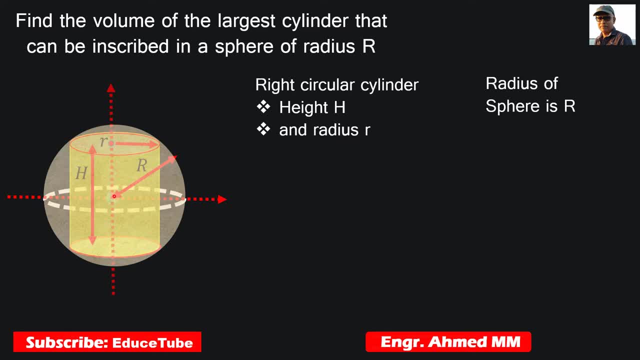 Now we are taking a right angle triangle from this point up to this center, then this h, so from here here and up to the center. So we take this triangle here. say here radius small r, and this is the- I mean sphere radius and this height. 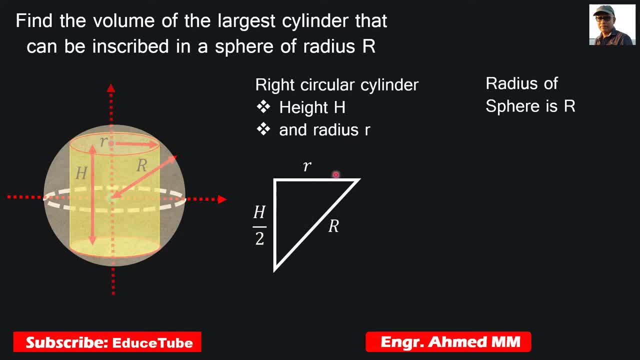 half of the height of the cylinder. it is h by 2.. So using Pythagoras theorem we can find the relations r square plus h by 2 square plus equal to capital R square. So next step we can write like this and then easily we can find r square equal to capital. 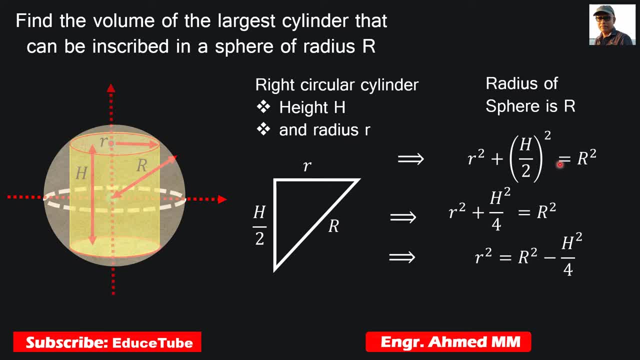 R square minus h square by 4.. Actually this equation we will use in volume, Because here there is a volume of cylinder. this is pi r square, I mean cross sectional area of this cylinder. say, if it is the area of this bottom circle, then multiplied by height it will be the 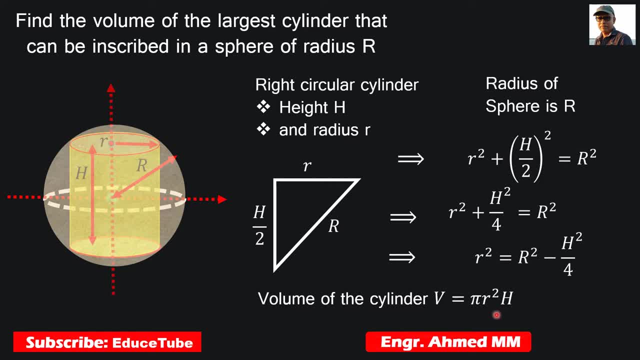 volume. But in the next slide here r square, we will replace this r square by this one r square minus h square by 4.. The reason is, once we get that equation we will do differentiations, Because we know to get the maximum volume of the largest cylinder we need to know. 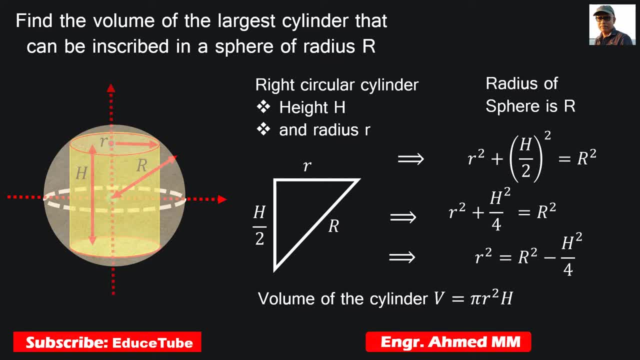 first derivative it is equal to 0, to be considered first. Then we'll check with the second derivative. either it is coming negative or negative, plus 0 to complete the double interior Ł using the second derivative. Either it is coming negative or negative, minus h2, and we'll be checking with the Diamond ofsimilarity. 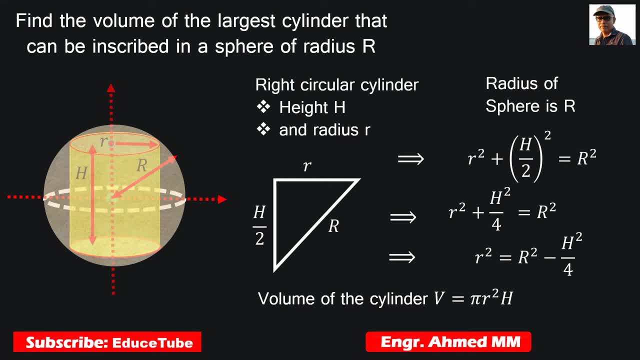 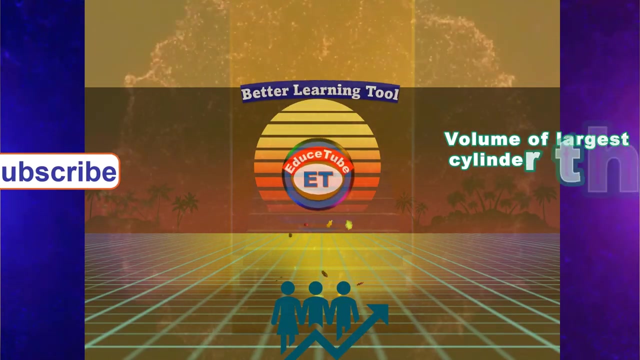 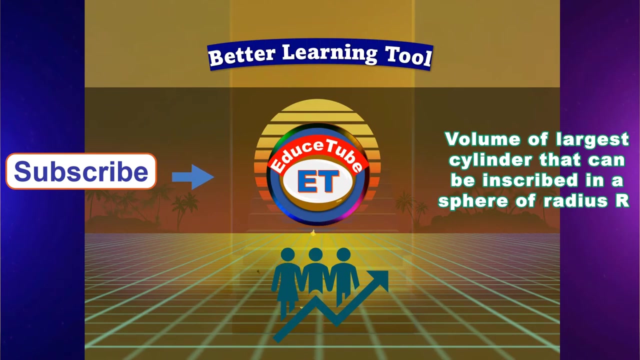 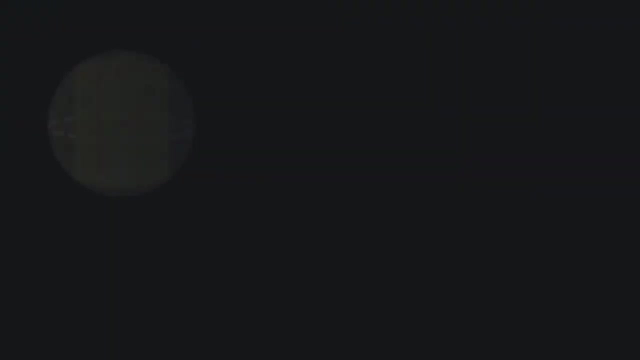 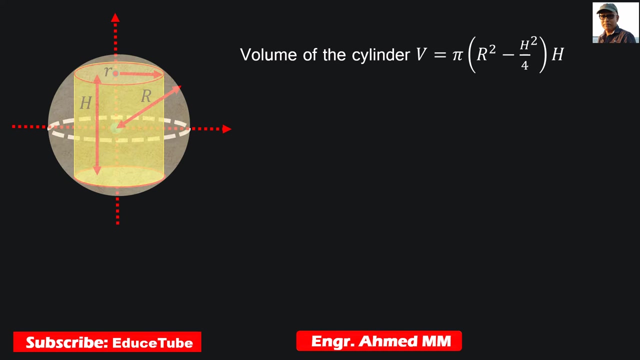 or not. if it is negative, then we will be sure that the volume of cylinders- larger cylinder a volume- will be maximum. so let's move in the next slide. as i said, our volume of cylinder equations will be pi? rs square- i replaced it by this one- and then h. 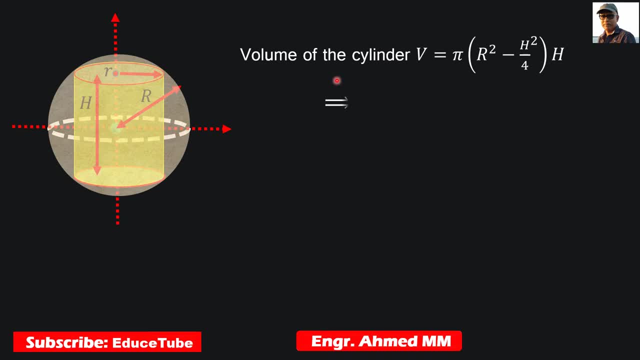 as i said, we have to do differentiations. why? to get maximum or minimum volume condition is first derivative equal to zero. so differentiating both sides of this equation- dv by ds equal to this, result will be like this. so dv by ds equal to this, result will be like this: 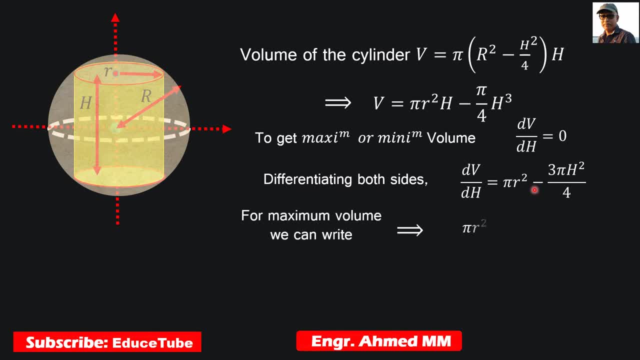 so maximum volume we can write because, as i said, this must be equal to zero. so this part, right hand side, we are writing equal to zero. so let's find a relation between h and r. so we got height of the cylinder equal to 0.2. 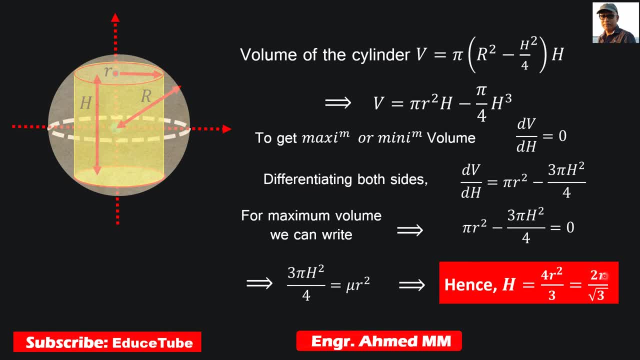 plus width plus height of the cylinder, we get 3. so this will be same like this as says for box problem. another, only about 2.54, will be z of a cylinder. this alone, that will be 0.5. guys. what is equal to z in this next slide? 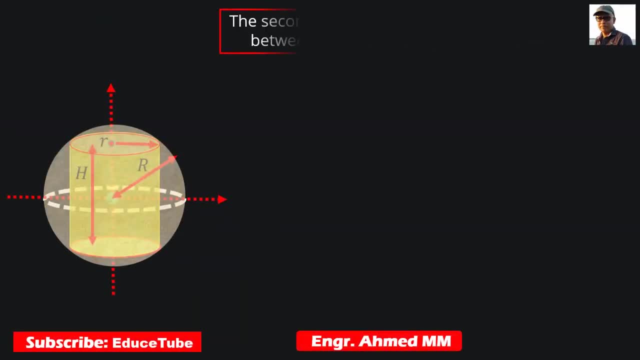 so that's the plan here. okay, so each section in the right hand side of the next hombres, Caribbean point, isiah 저는. So, second derivative, we test to distinguish between maximum and minimum, to be sure with either it is maximum or not. So our condition is already we have taken this first derivative 0. 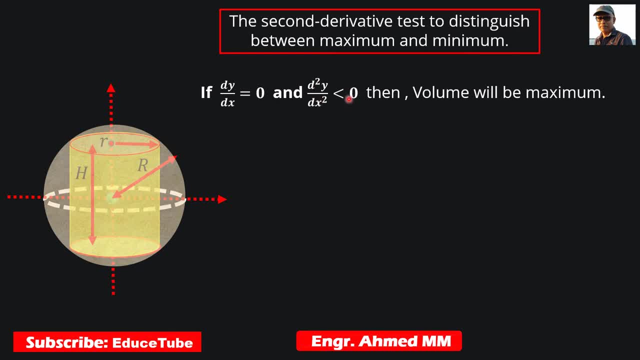 and second derivative, right now we will do to see value comes negative or not, to be sure, with that volume will be maximum. So let us do that, So differentiating both side. with respect to H, which one? This equation Already we got this. 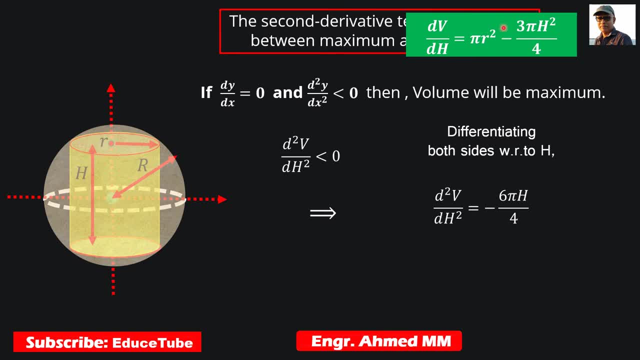 equation in previous slide. So we are differentiating this and we get this second derivative. So once we get second derivative, we get this second derivative. So we need to replace this H by equal to 2R, by square root of 3. These relations we got in. 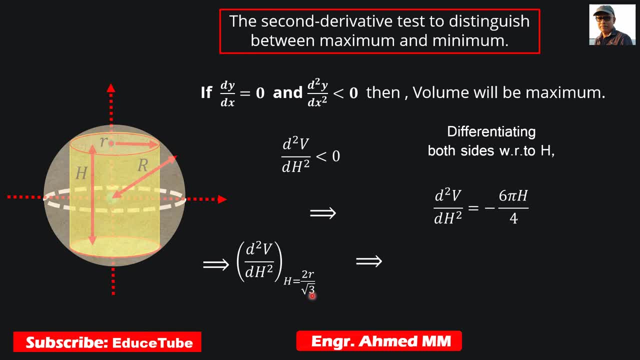 previous slides. Now only our task is to replace this H by this. So we replaced it and at an end I found minus square root of 3 pi R. It is negative, So it is less than So, we are sure. now. 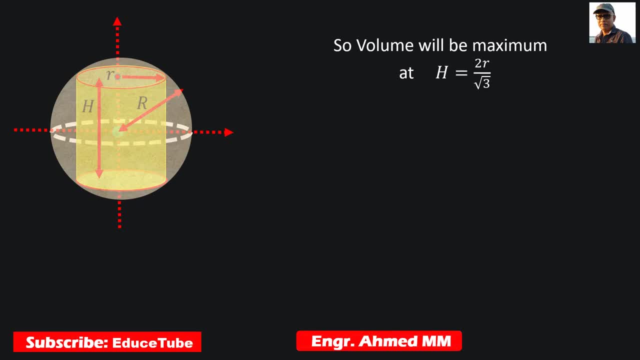 and then final. So we assume now that it must be 0. So we assumed that H, what we want is Hinter constant plus pi, R and abandon, and there is thespite in that. So we are sure we are given. you will not take the second derivative다가. 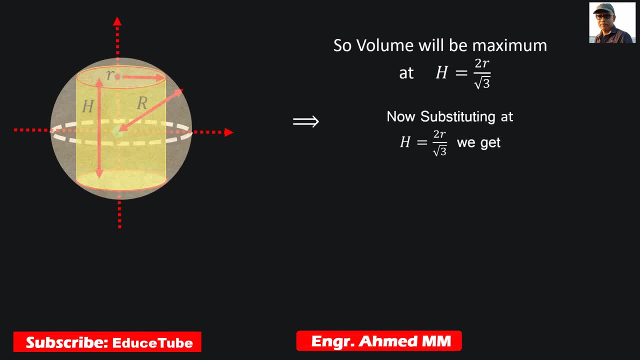 derivative with respect to this H by the square root of 3.. So the volume will be7.. So we are sure now that it will beасure. Volume will be math in match. so we are sure now, volume will be maximum at糖. So H equals to 2R by square root of 3.. Then volume with value equals value gained, It will robots volume at H equal to 2R divided by square root 3.. We are sure now because already we got second derivative negative. 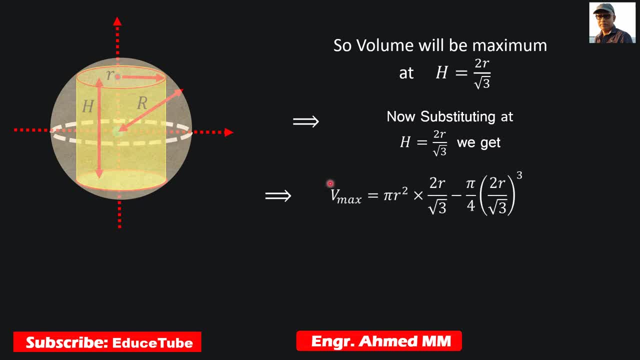 root of 3, we get maximum volume already. we got this equation in previous slide. only we are replacing this h by this, because this was our volume equation, so h, we are replacing this. at an end, we got 4 pi r cube by 3 square root of 3, this is the result we were expecting.